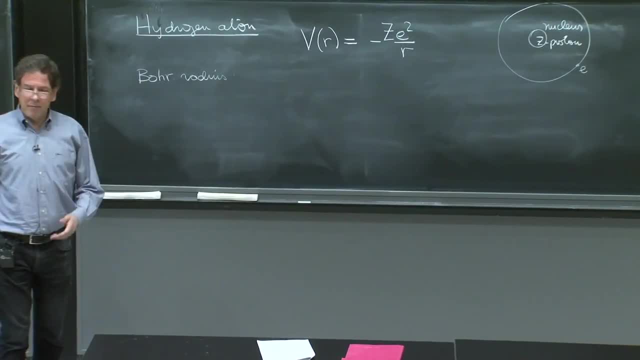 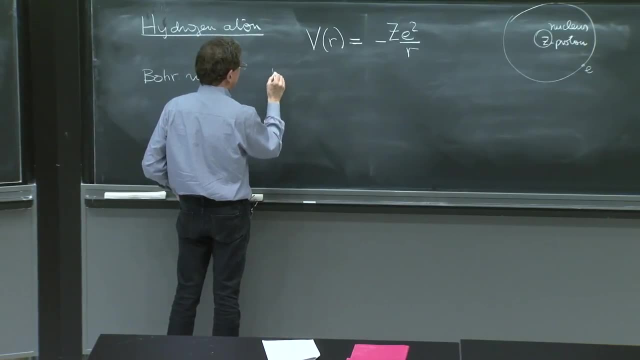 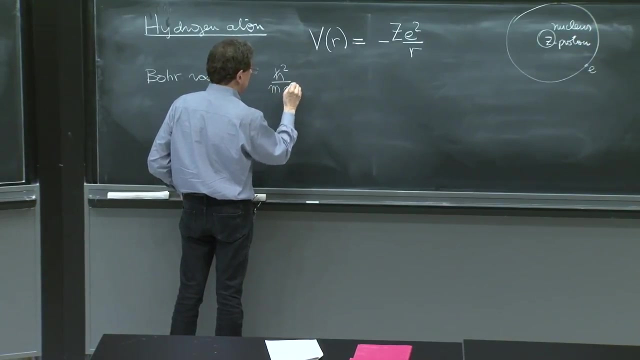 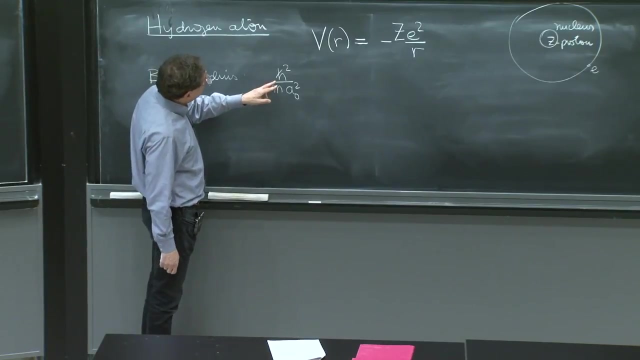 And So one way of calculating the Bohr radius is to just think of units and think of energy. Energy goes like h squared over ma squared. This has units of energy. You remember p squared over 2m And p is h over distance. 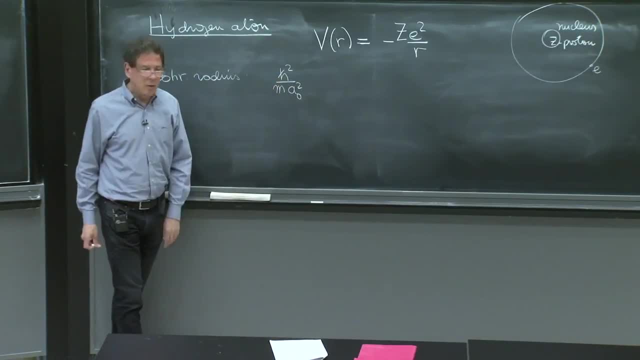 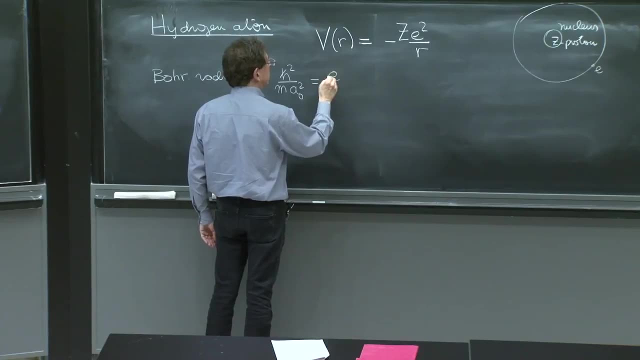 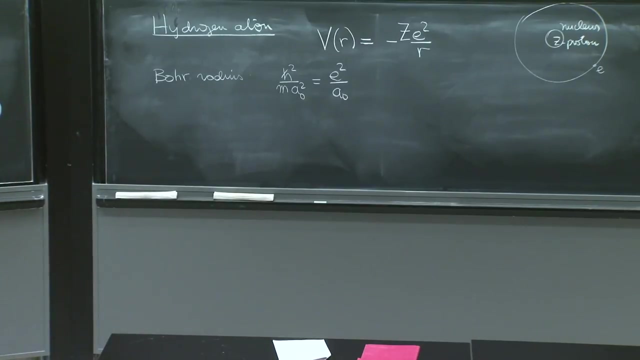 So if you have a Bohr radius a0, this quantity has units of energy, But a potential has units of energy, And we just put e squared over a0. So this is a consistent equation between two quantities that have units of energy, from which you 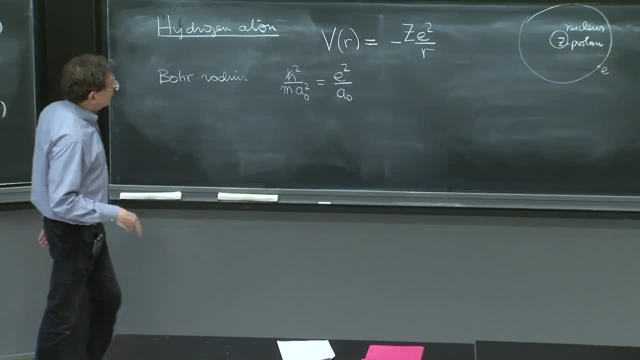 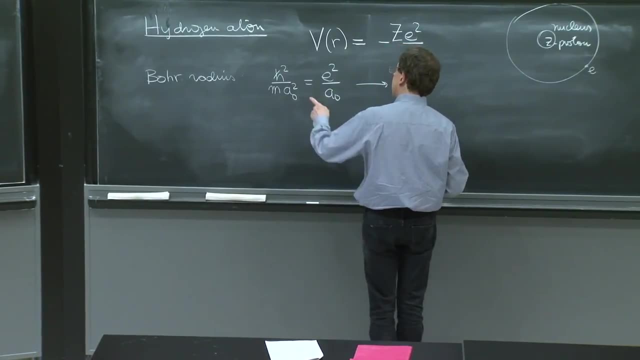 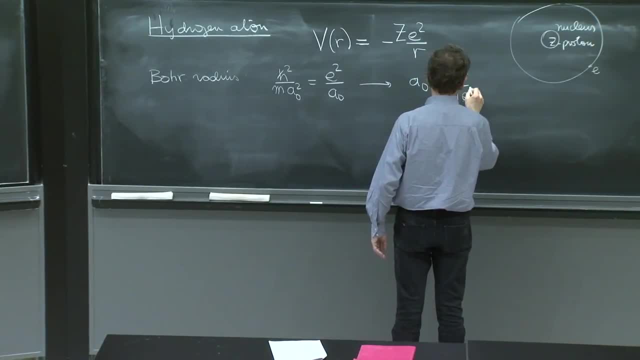 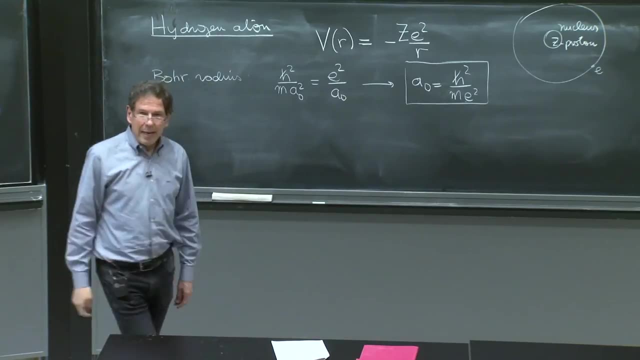 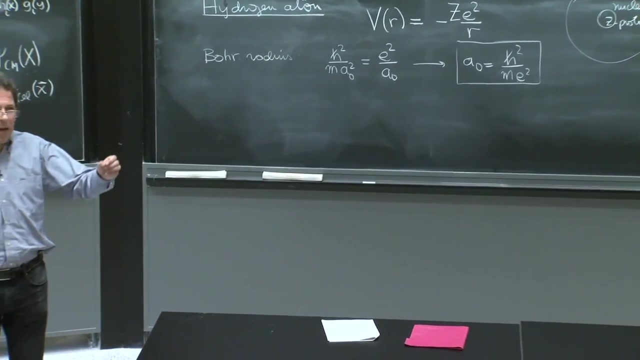 h squared over m, e squared. It's a very simple and nice constant. It's the Bohr radius, Intuitively, one thing that you should remember: e is appearing in the right place And you can imagine if the strength of electricity. 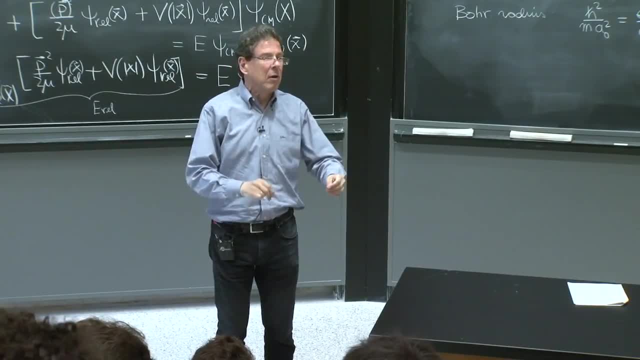 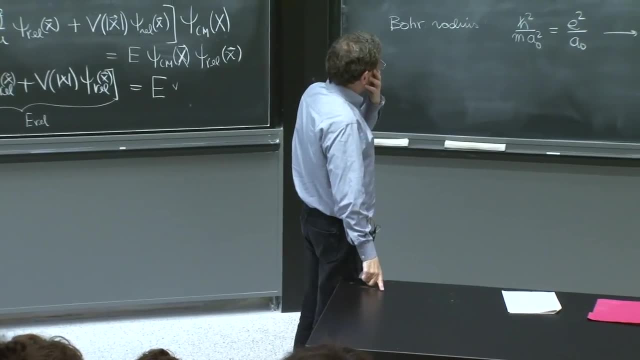 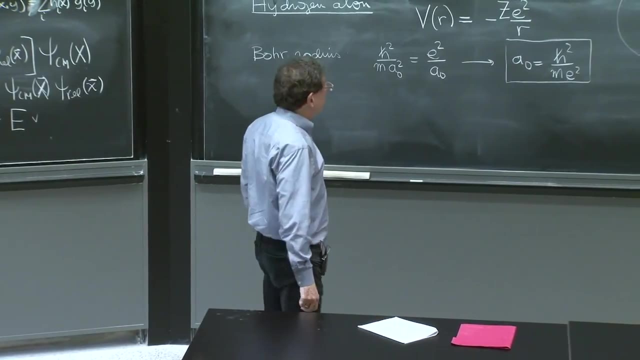 was weaker and weaker, like setting e going to 0, the atom would become bigger and bigger. It would just not be able to hold it. So it's reasonable to expect this to happen. So at this moment we can calculate what this is. 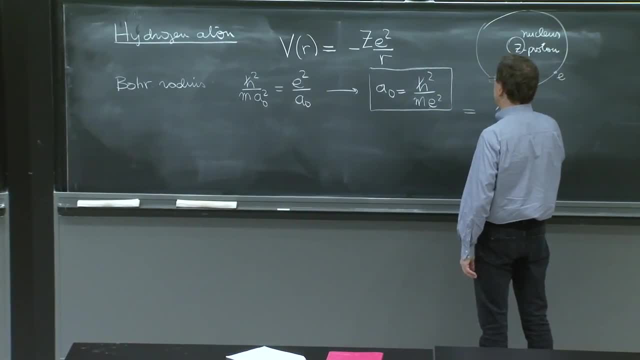 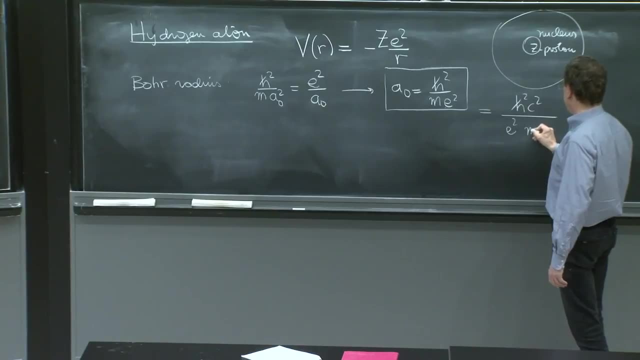 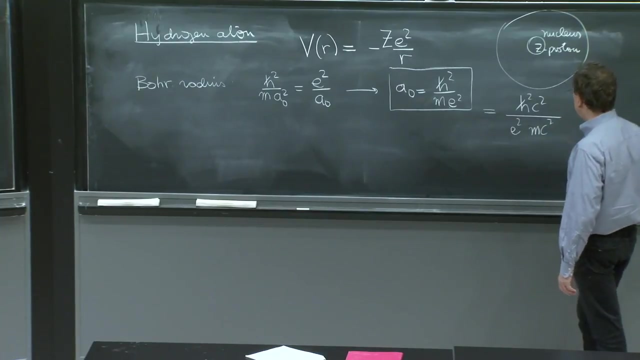 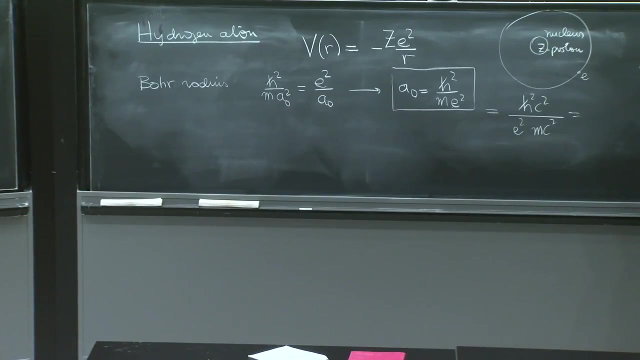 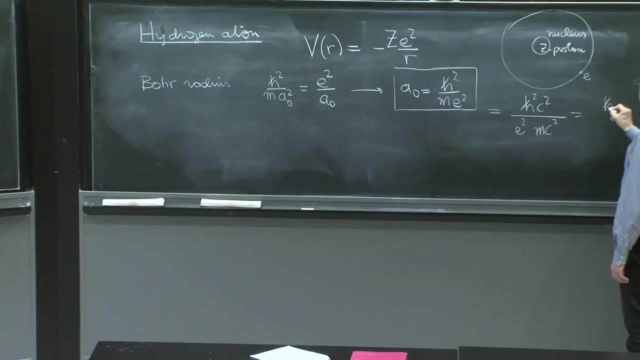 at least estimate it. And for that we multiply by a, c squared, e squared over mc squared, And then we recall that e squared over hc is about 1 over 137.. So we'll write this as hc over e squared over hc times mc. 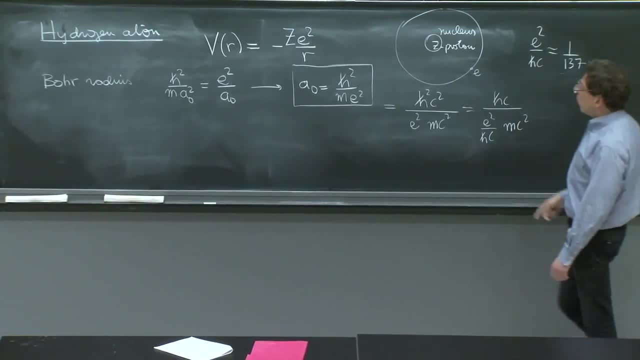 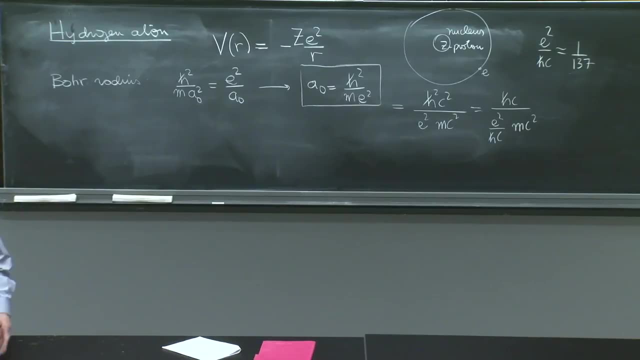 squared Now in here. what mass is the mass that we should put? I will not be all that careful. It should really be the reduced mass, But it differs by a factor of one part in 1,000 or less even from the mass of the electrons. 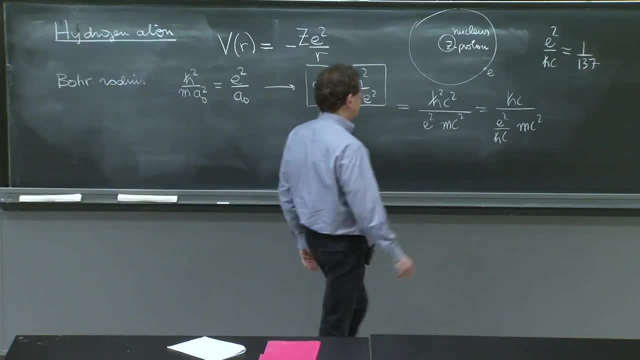 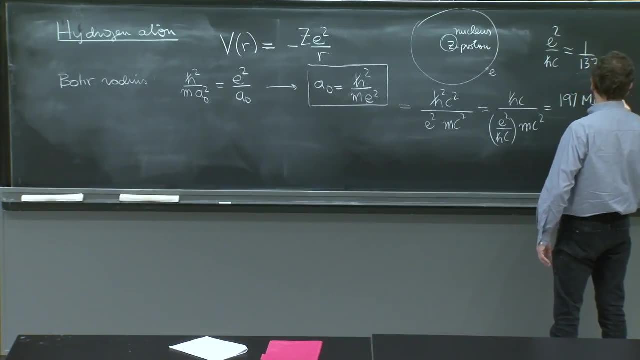 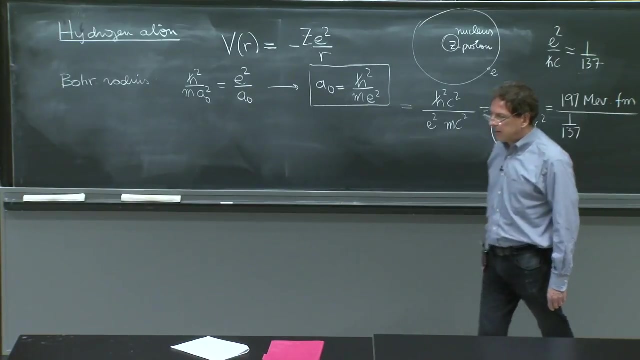 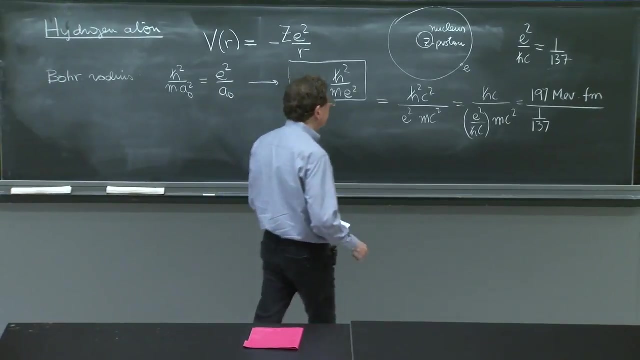 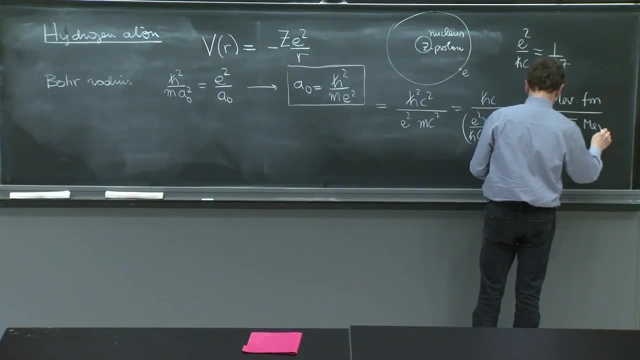 So I'll put just the mass of the electron. This is about 197 MeV. Fermi, This is 1 over 137.. And for the electron it's 0.5.. It's 0.5 times 10 to the 6 EV: 0.5 MeV. 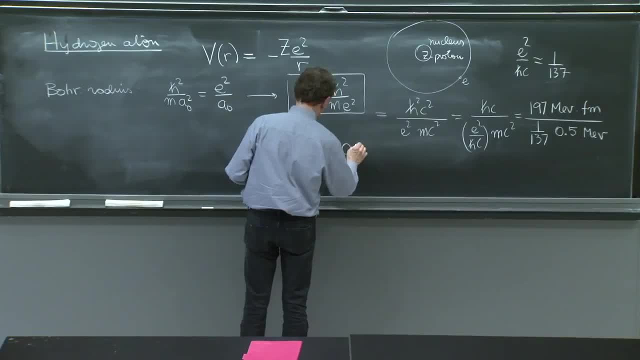 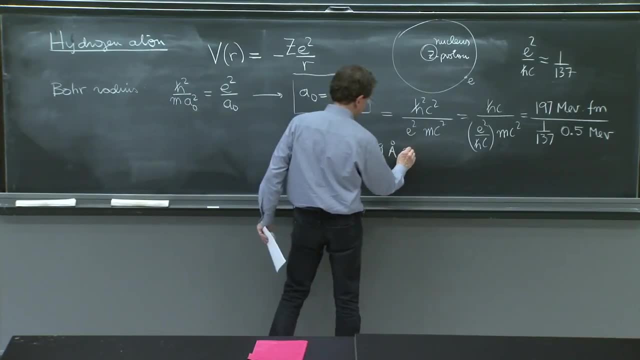 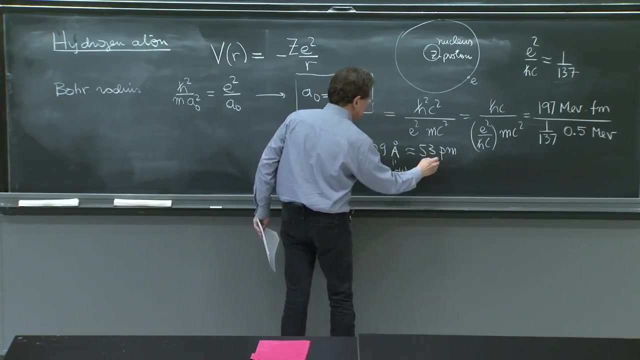 I won't run the numbers. The answer is about 0.529 angstroms, which is about 53 picometers. Angstrom is 10 to the minus 10 meters. Picometer is 10 to the minus 12 meters. 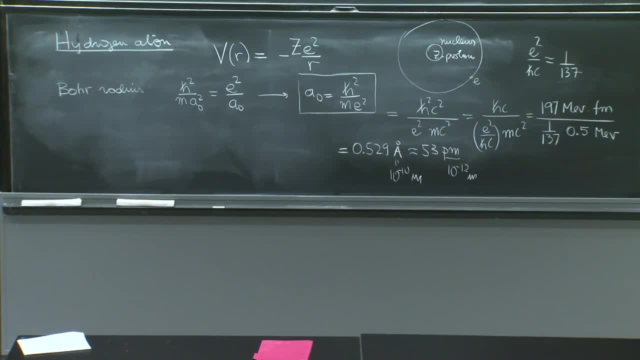 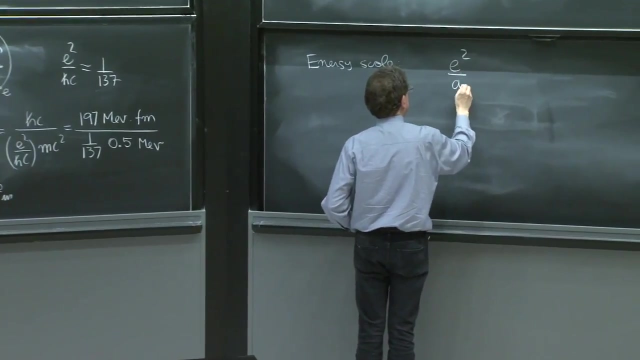 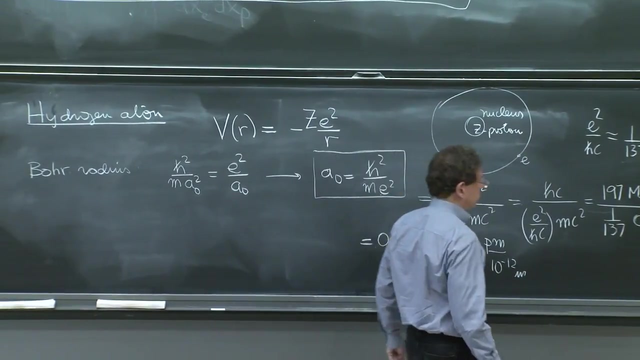 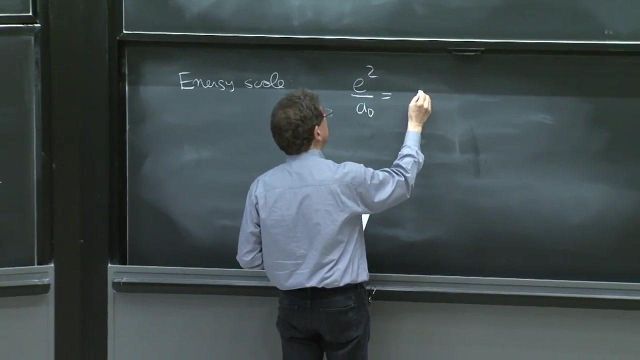 So that's a length scale. you've seen several times. There's an energy scale that is famous too, And that's e squared over a0. Because energy comes here and the energy scale is e squared over a0. So you can substitute what a0 is, because you know it already. 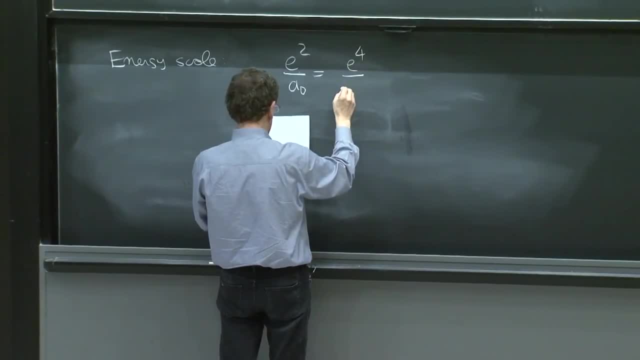 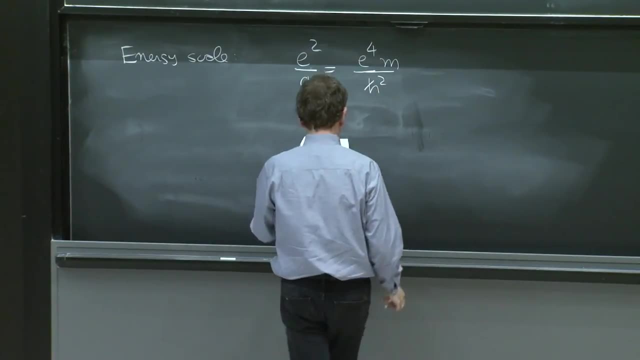 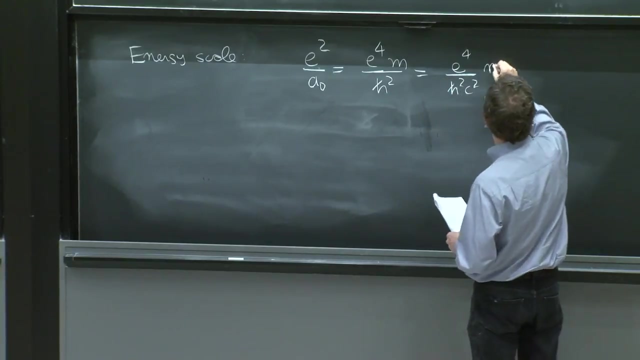 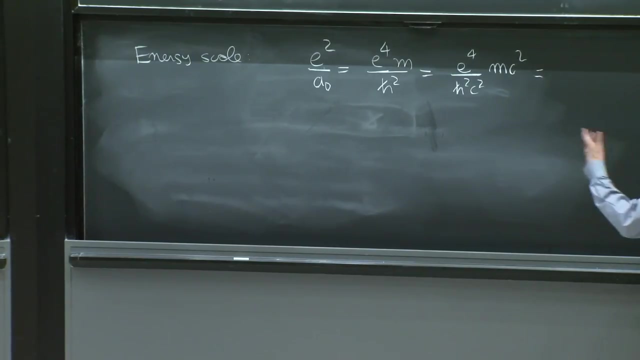 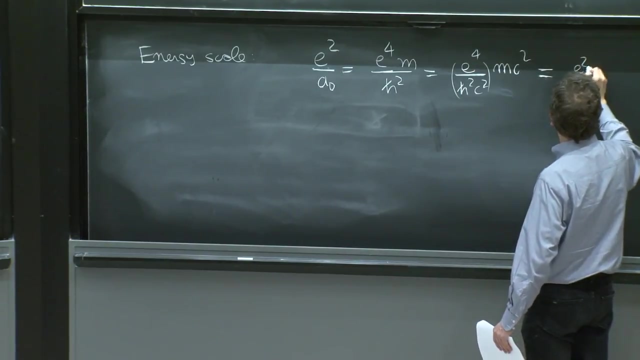 And you get e to the fourth over m, over h squared, which is e to the fourth over h squared, c squared times, m squared, mc squared. And you see, it's kind of nice to see these quantities appearing, because here you have e squared over hc squared. 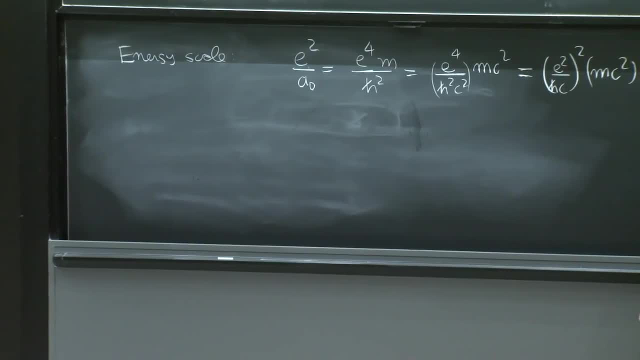 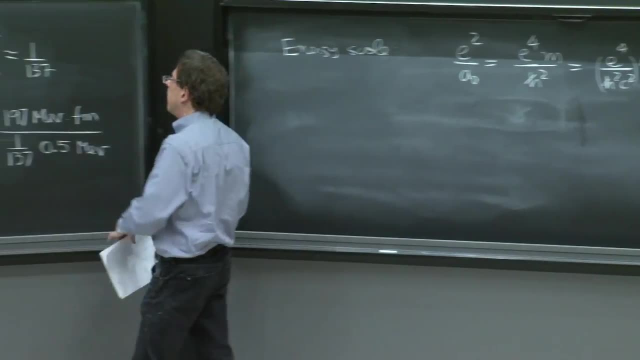 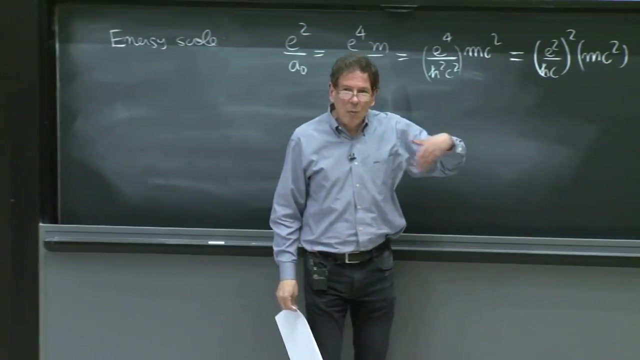 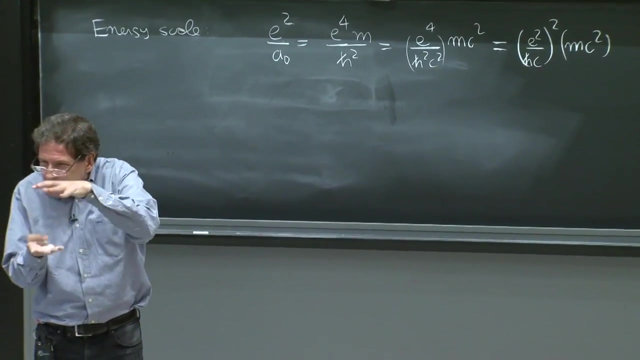 times mc squared. So the typical energy of the hydrogen atom is the fine structure constant, sometimes called alpha squared times an energy And what energy is available in the problem, The rest energy of the electron. So if the bound state energy should be something, 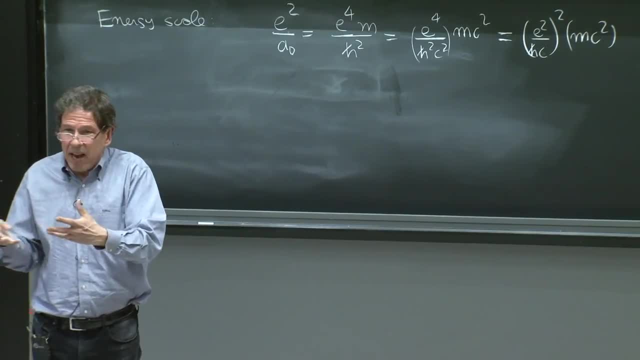 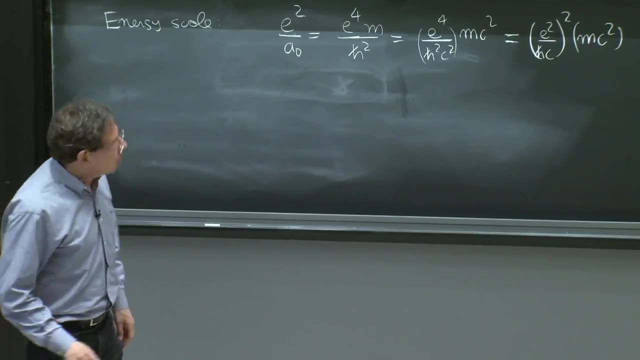 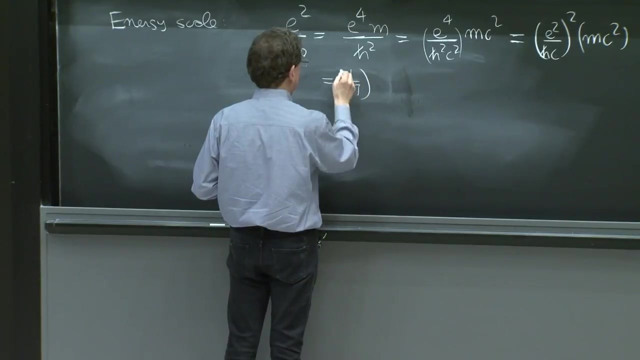 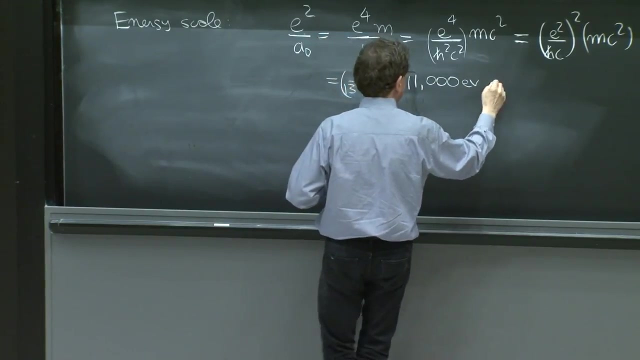 it should be a number proportional to the energy that the problem already has. And the problem has one energy. The rest energy, The energy of the electron, So it's not too surprising. So it's 1 over 137 squared times 511,000 eV. 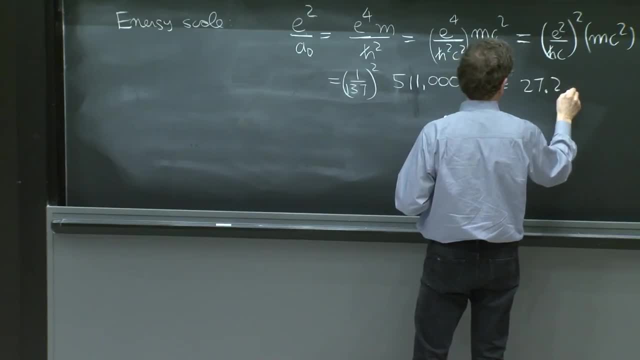 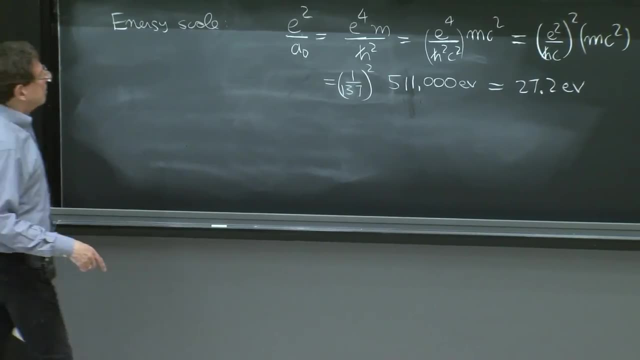 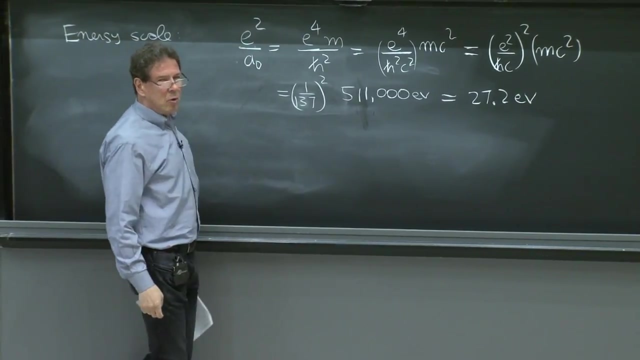 And that's about 27.2 eV. And the reason this may sound familiar is because the true ground state energy of the hydrogen atom is the energy of the hydrogen atom. The hydrogen atom is this number divided by 2, which is 13.6 eV. 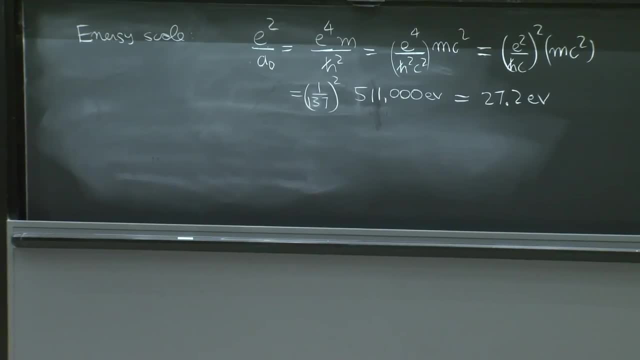 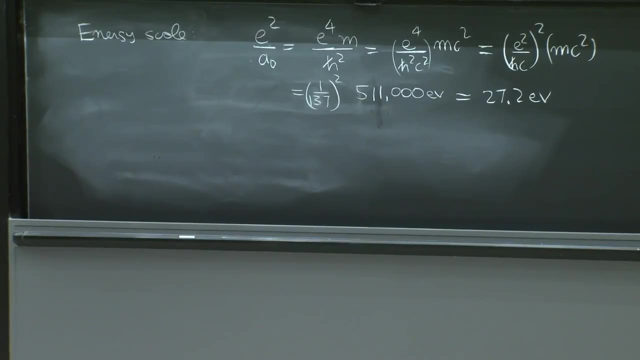 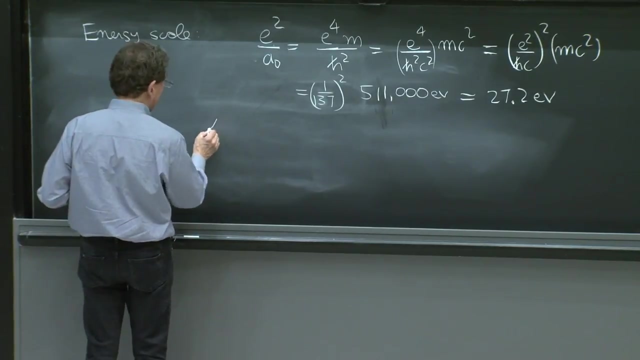 So of course you would not know at this stage because you're just doing numbers. I may remind you of things you did a long time ago. in this course You calculated a couple of other constants And you show that alpha again, the fine structure constant. 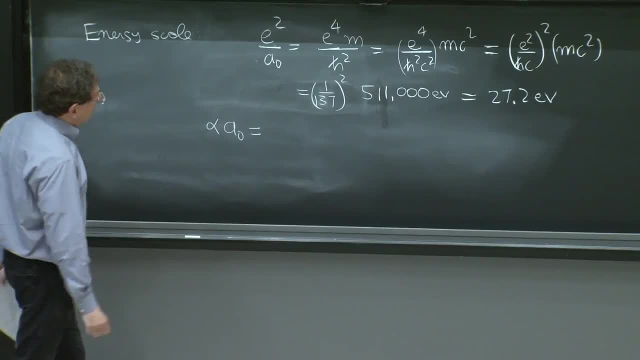 times a0.. It's very interesting And this is going to be what you call the Venro-Wilhelian factor. But it's not just the value of the value, It's the value of the temperature of the energy. So it is going to be positive. 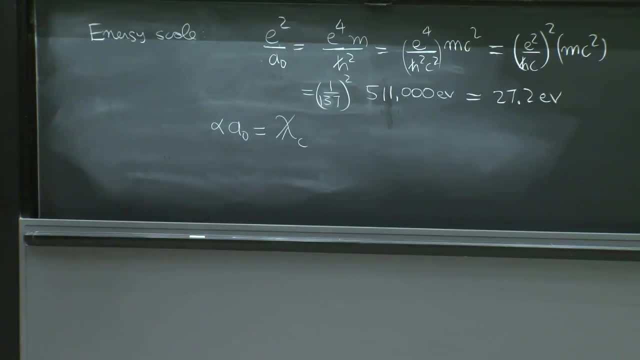 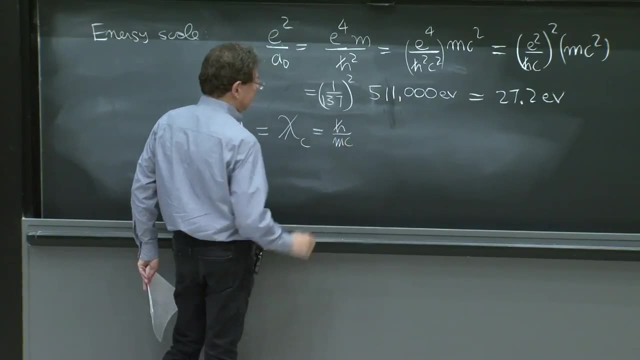 It is going to be negative with the temperature. So it's 1 over n squared, So I can convert that to positive And I can convert that to negative, And that is going to be negative. So if I go ahead and multiply that with the negative, 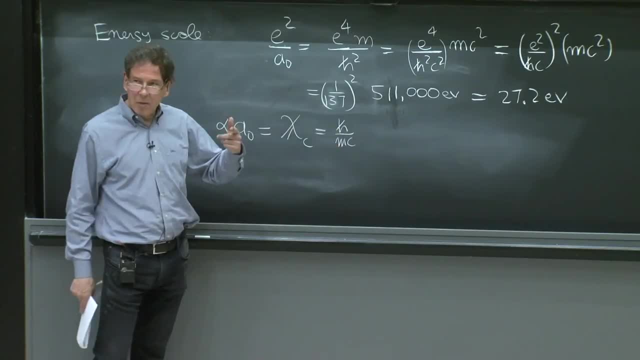 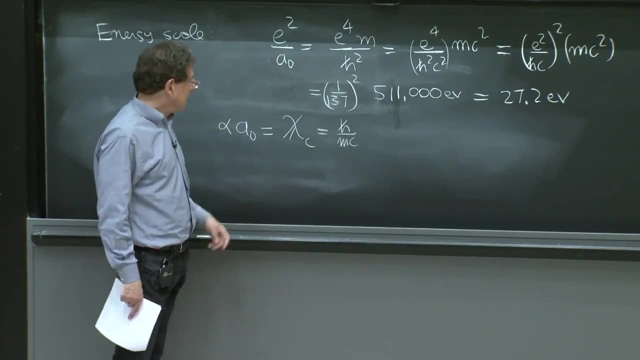 I can say that it's 1 over n squared over n squared, And that's good because it's negative, But that's also negative. It's negative, What's negative, And wavelength is h bar over mc, And that's what alpha times a0 is. 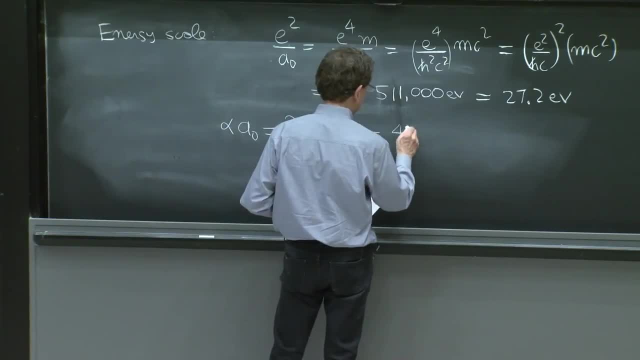 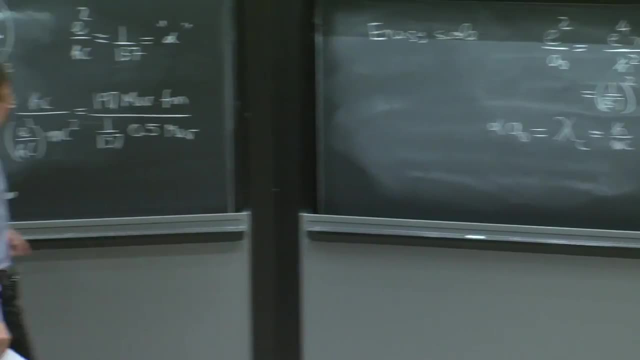 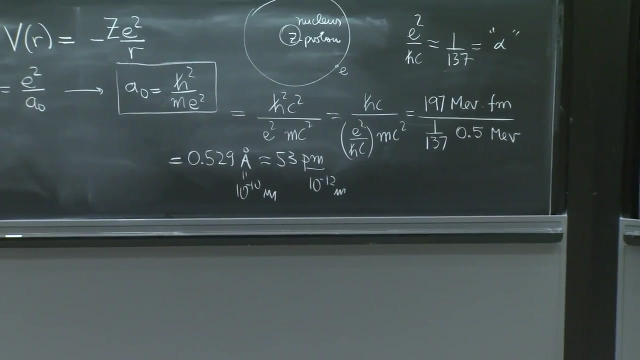 And that quantity is about 400 Fermi. It's already much smaller than the Bohr radius. It's smaller by 137 from the Bohr radius. And then, if you do alpha squared, a0, that actually was the classical electron radius.